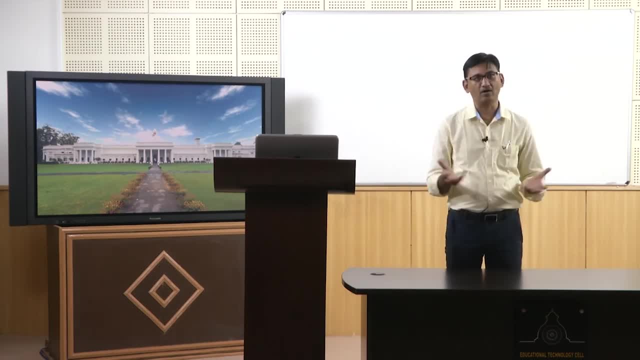 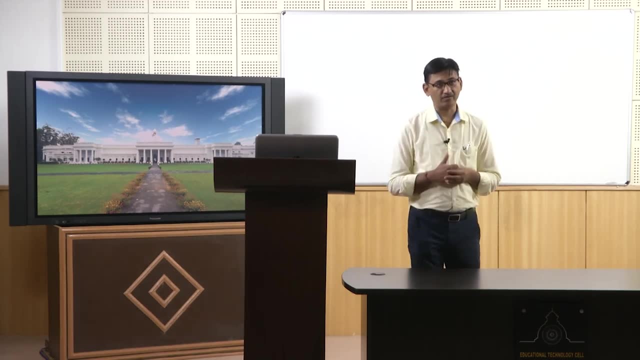 type of bonding, okay, in this case covalent bonding with all the carbon atoms. Then it is a new form of different allotrop of carbon, which is diamond and it is a hardest material known to man. okay, so just by changing the bonding between the same type of atoms. 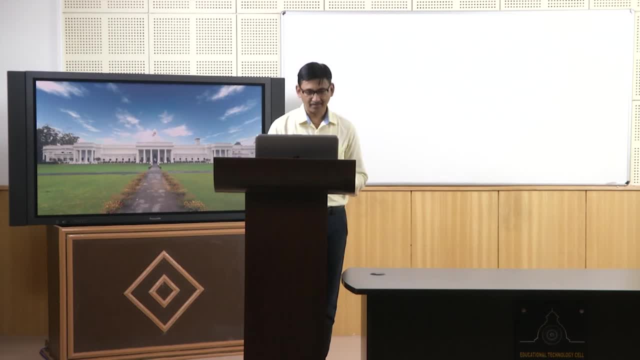 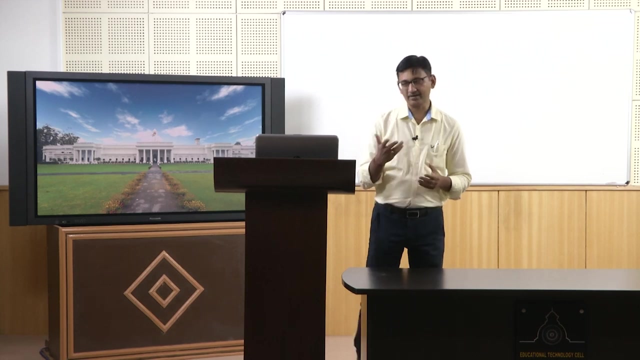 okay, we have changed the properties to such an extent. okay, if you compare now between, let us say, metals and ceramics, okay, one, two class of materials widely used. okay, metals have slightly weaker bonding. okay, and their properties are decided by what type of bonding they have, which is called metallic bonding, and ceramics have either ionic or covalent. 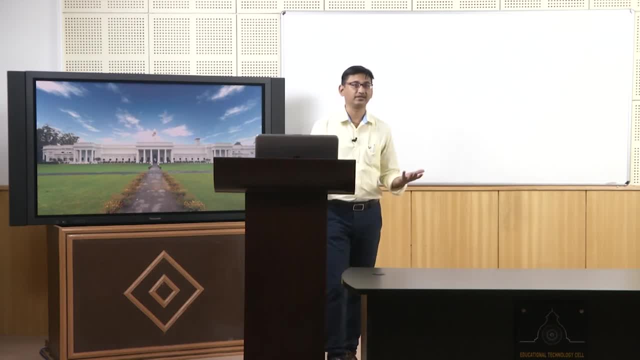 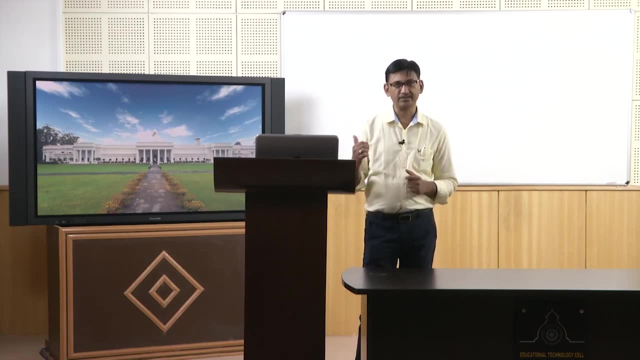 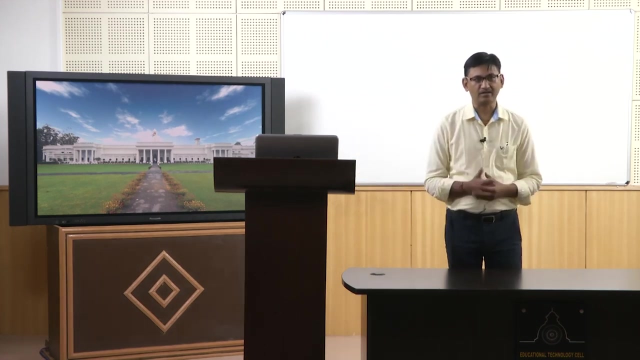 bonding: okay, and their properties are decided because they have this type of bond and what is the bond? strength and so on. okay, so we will see this type of bonding. first, we will see the atomic structure. okay, which is basically your 10th class physics, or up to 12th class. 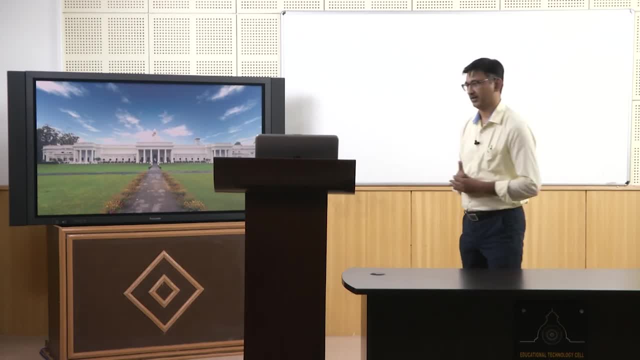 physics. Okay, just recap of all the ideas which we have already. you must have seen at some, in some other, in 10th or 12th, okay, so let us start with that. So, atomic structure: if you see, okay, an atom consists of nucleus, which is which has proton. 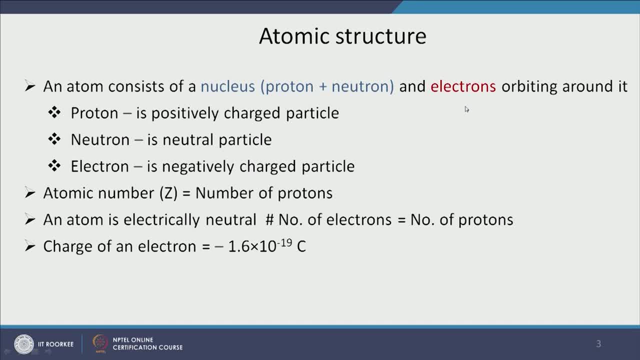 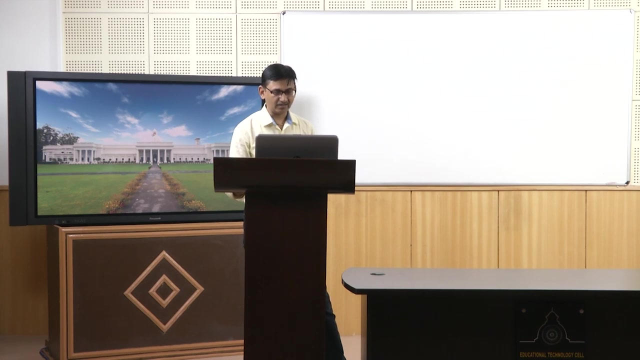 and neutrons and electrons orbiting around it. okay, proton is positively charged particle, electron is neutral and electron is negatively charged particle atomic number is equal to number of protons. and because it atom is electrically neutral, okay, the number of protons will be equal to number of electrons, and the charge of an electron is given here in coulombs atomic. 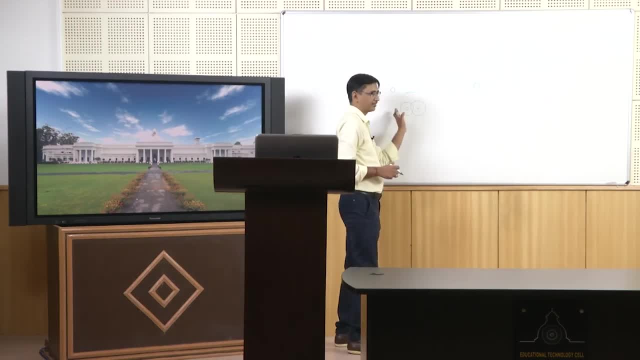 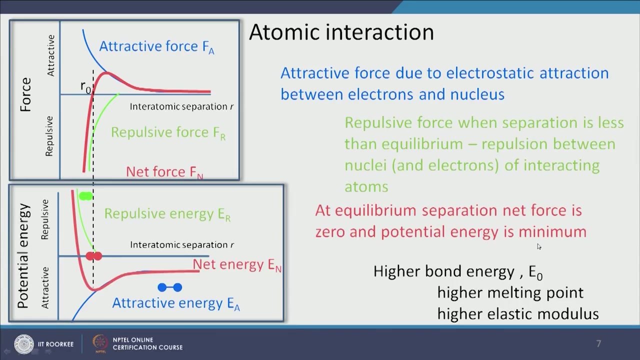 if you take them far apart, the electrons of this atom will be attracted by the nucleus of the other atom. okay, So these are the two forces which is going to act at equilibrium separation. net force is 0 and potential energy is minima, as we just discussed. okay, so now the there is one. 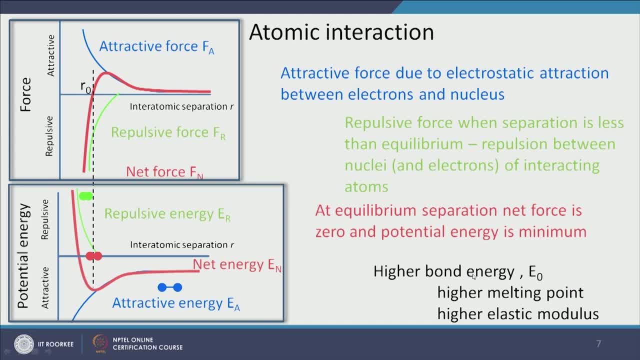 term we are bringing here, which is called bond energy. okay, so the bond energy is the energy which is given by where the minima is there. so if I measure from this minima up to the 0 energy, okay, So this is my E naught. okay, this is the E naught. okay, measurement from x axis to the 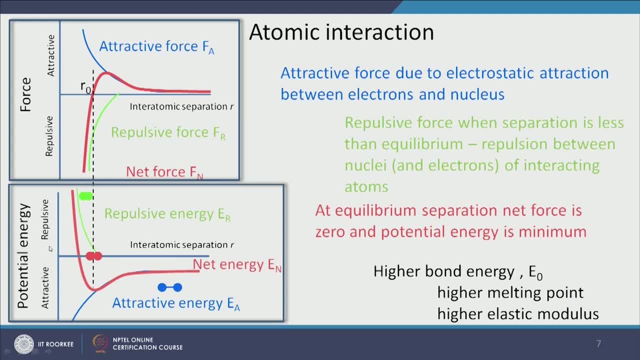 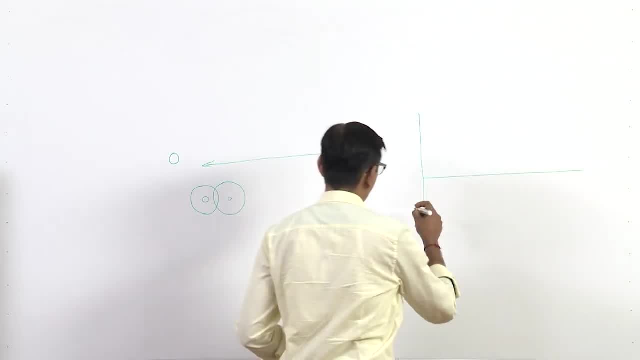 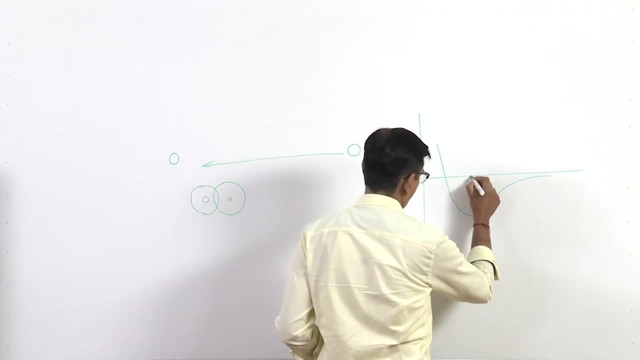 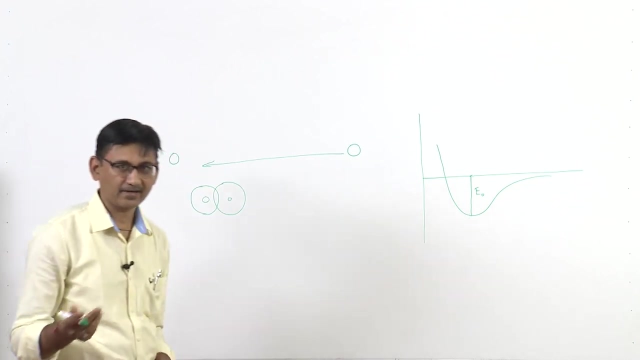 minima here, so I can have different energies depending upon the, for different materials or different atoms. okay, so maybe in one case I may have energy like this- okay, and this is what I am calling as E naught- Okay for another material or of another type, another atoms. maybe the energy is something. 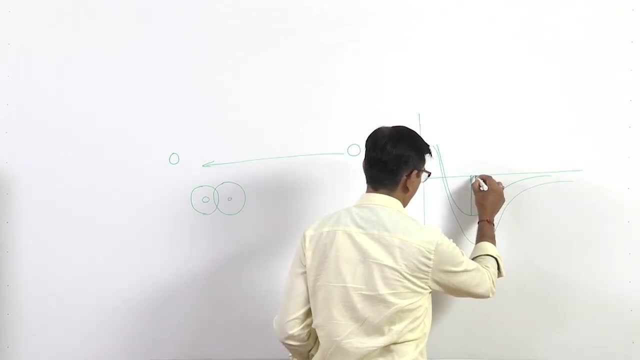 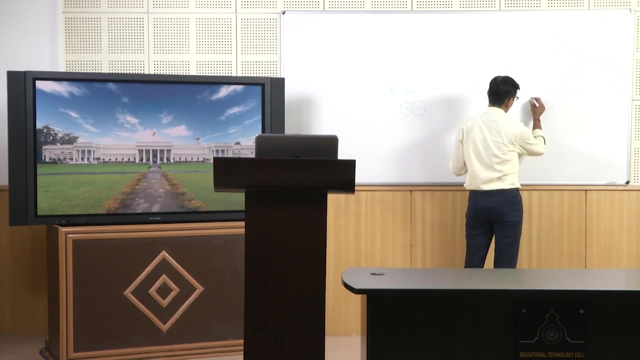 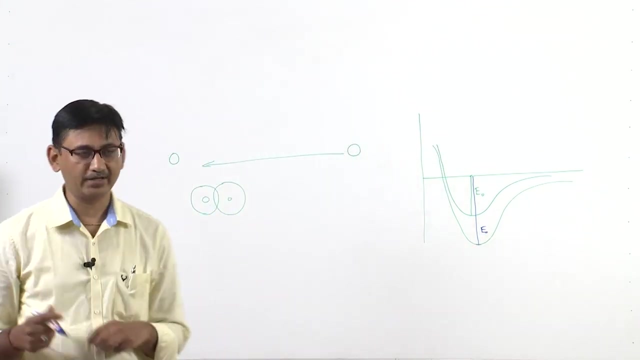 like this: okay, so now in this case, my energy has increased. okay, so let us see if I draw it here again somewhere here. this is now E naught for another material. okay, so now you can see that for this material the energy is even lower. 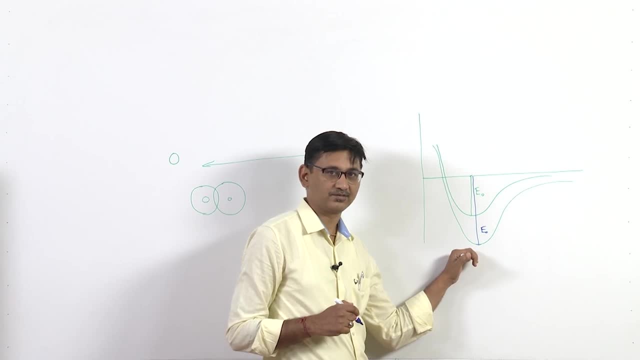 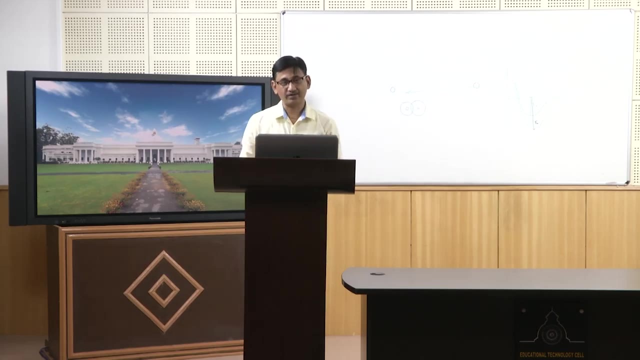 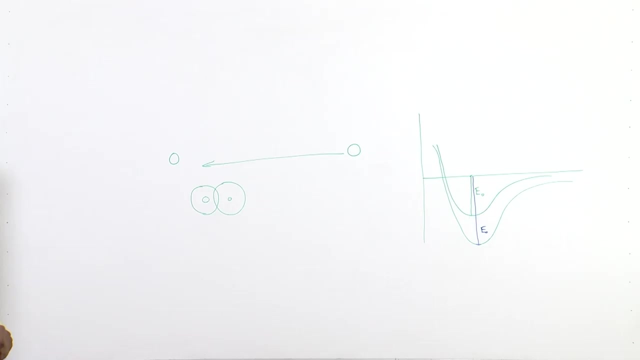 Okay, so the bond strength of this material will be more than the bond strength of this material. okay, and that is going to affect the properties of the material. okay, so you can see that if I have higher bond energy, E naught, I will have higher melting point. 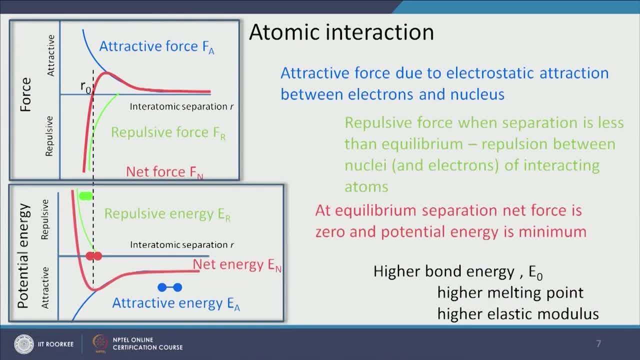 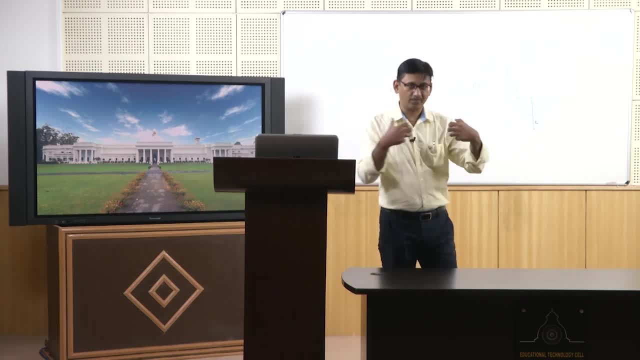 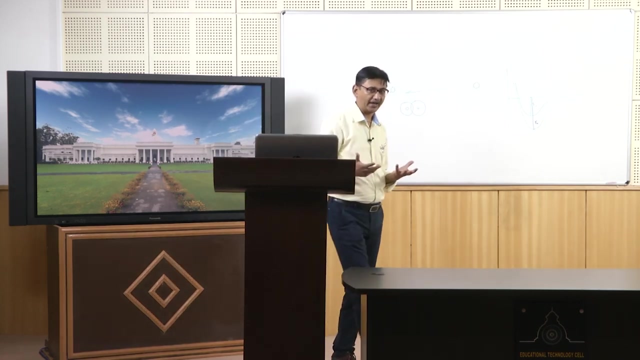 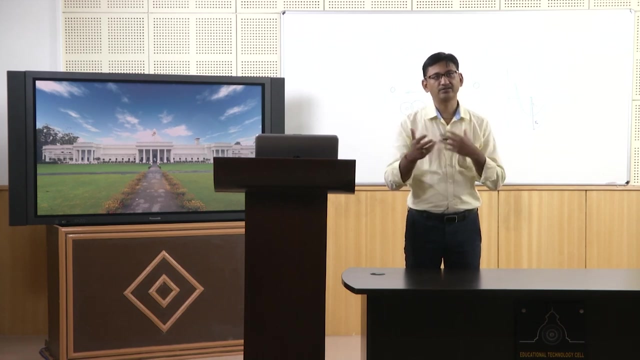 okay, it will be more difficult for me to break the bonds and take it into the liquid phase. I will have higher elastic modulus, okay. 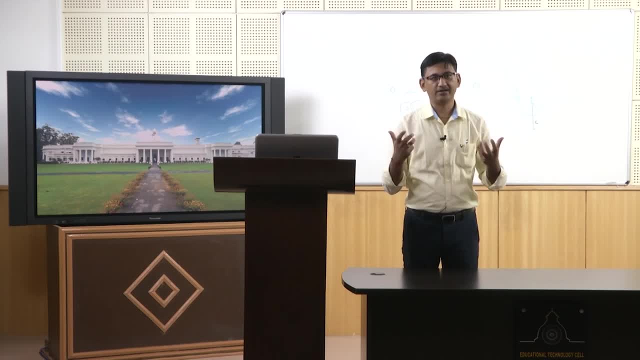 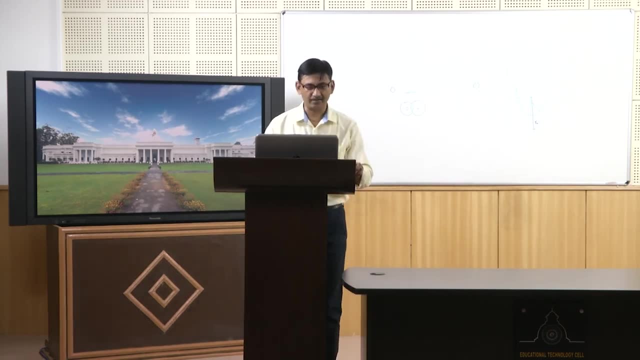 but the bonds can be of different types. okay, so there can be. you can classifying them into two categories here. one is primary interethnic bonds, which is ionic, covalent and Metallic, and secondary bonds, which are under wall forces. 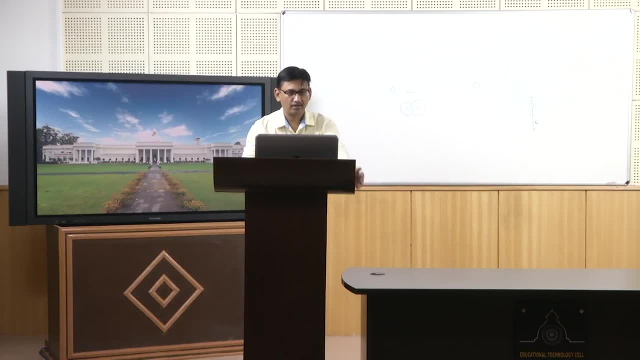 and hydrogen bonds. okay, now if? Now, if we try to understand what do we mean by ionic bonds? okay, the ionic bond means you have two ions which are interacting. So, for example, usually these ionic bonds form between metallic and non-metallic atoms, and metallic atoms give valence- electron- to the non-metallic. 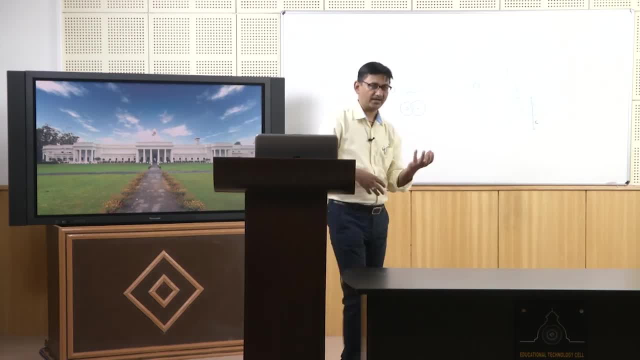 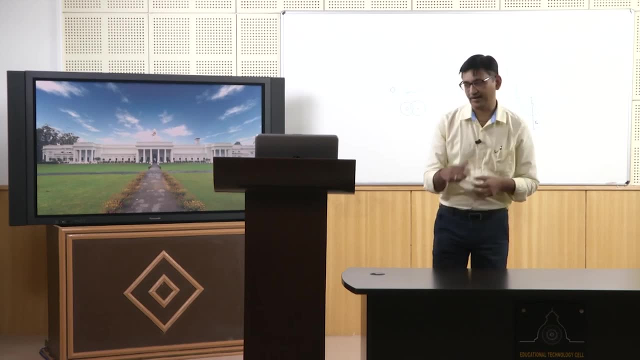 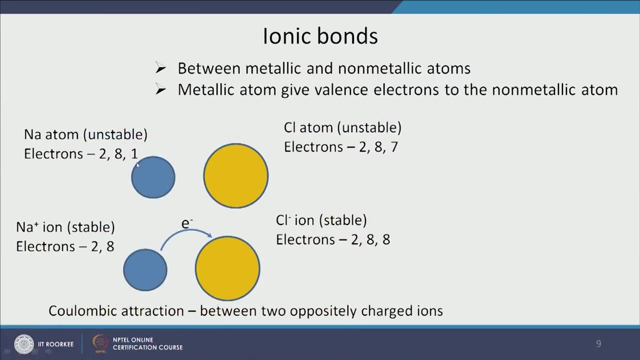 atom. So by giving electron it becomes an ion, and by accepting an electron by non-metallic element it becomes another ion. So, for example, if you see the sodium atom, it has unfilled shell, So its electron configuration is 2 at 1, 2 electron in the first shell, which 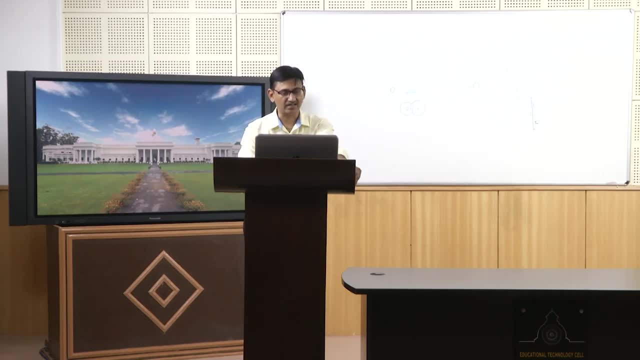 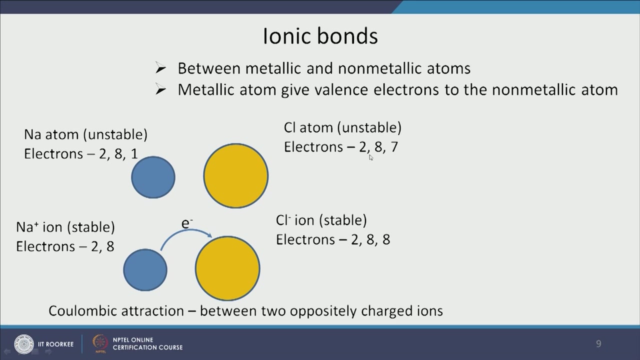 is K shell, 8 electron in the next shell, which is L shell, and then in M shell you have 1 electron. It needs 8 electrons here. Chlorine atom: if you see it has 2 at 7 electronic configuration: 2 in the first shell, 8 in the next shell and then 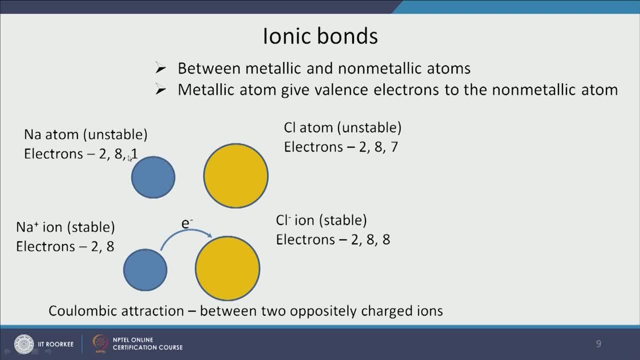 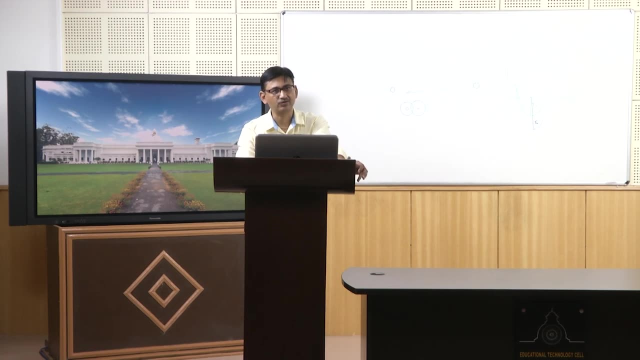 the 7 in the third shell. So if sodium gives 1 electron to chlorine, it will become stable because it will have all the shells as filled. Similarly, chlorine will also get 1 electron to fill the shell of the chlorine atom. So that is what they will do. Chlorine ion is a positivo charge. Now this is an electron ion. You can see that this is a isotropic ion. It is a positive charge, So this is an electron ion. It is less than that. So you will see that these 2 ions are of 4 electrons. Now this is a neutral charge. It is a neutral, beneficial situation for both the atoms. One atom will jump from the sodium, go to the chlorine, So now it becomes Na plus ion, because it has given 1 electron, So now it is a positively charge. 1 extra proton is there now which make it positive. 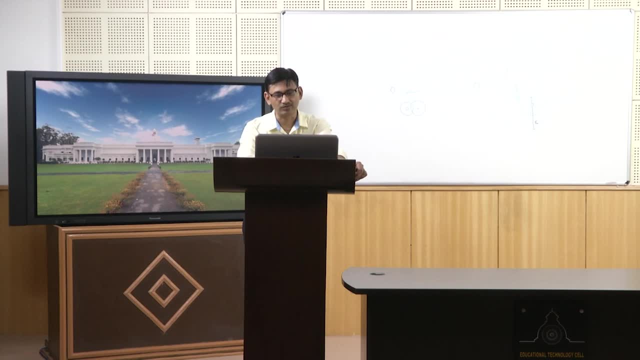 So it is 2,. the electronic configuration is of this ion is 2, 8.. Chlorine has accepted 1 electron, So now it is negative charge. This is a neutral charge, So it has also given 1 electron here. Now it will jump from the sodium to the chlorine ion. 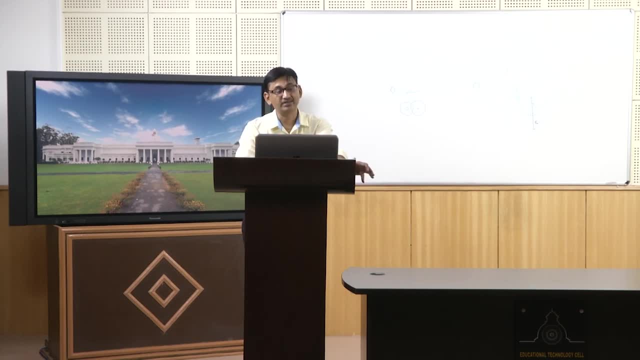 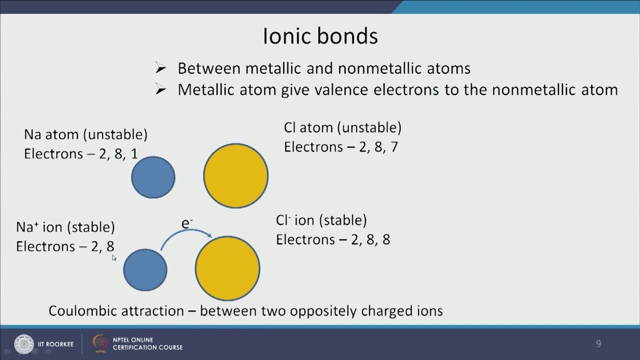 So now it become Na plus ion, because it has given one electron. ok, So now it is a positively charged. one extra proton is there now which make it make it positive, So it is 2. the electronic configuration is of this ion is 2- 8 chlorine. chlorine has accepted one electron. 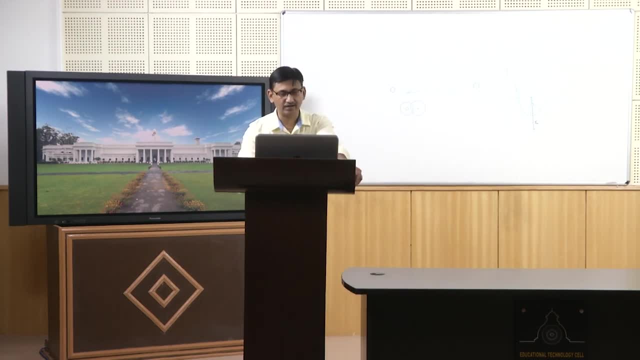 ok, So now it is negatively charged because the electron one has one. there is more, one more electron than the protons. ok, So now and now the electronic configuration is 2, 8, 8 and because of this positive and negative charge, there will be a coulombic. 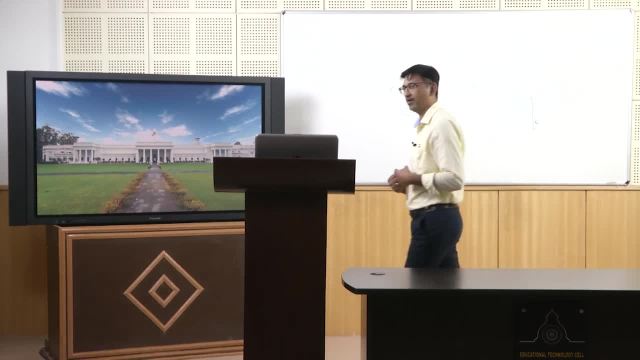 interaction between the two ions. ok, and that is what bonds them. ok, That is a very good situation for them. ok, giving each other one electron: ok, one electron is transferred from no sodium to chlorine, and then you have some attraction because they are now Oppositely charged particles, charged atoms. ok, If we come to the next type of bonding, 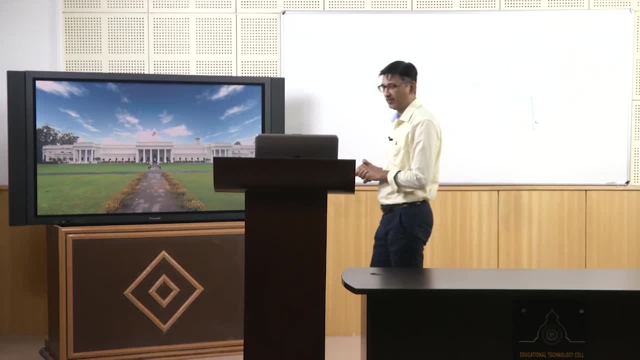 which is covalent bonds. in this type of bonding, atoms share. they do not give permanently one electron, but they share all the time. ok, So it is a sharing kind of relationship between the two atoms. ok, So they share their valence electrons to get a stable configuration form. 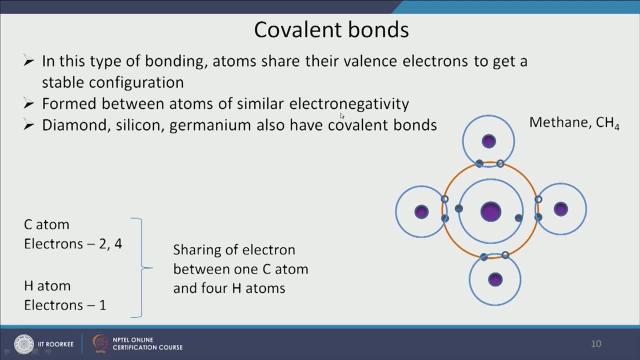 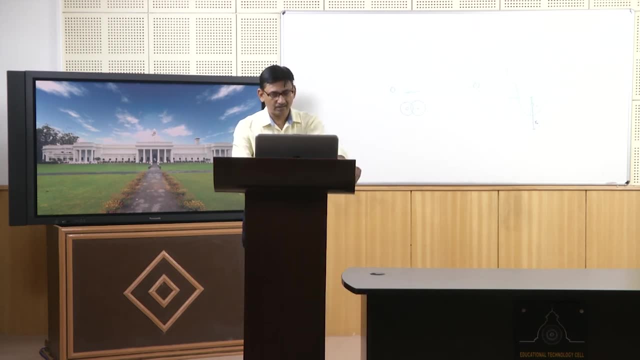 between atoms of similar electronegativity. diamond, silicon, germanium also have covalent bonds, ok, and that is that is what gives them sometime very high hardness. for example, diamond is the very hard material, ok. So carbon atom has electron configuration of 2 and 4. ok, and hydrogen atom, of course. 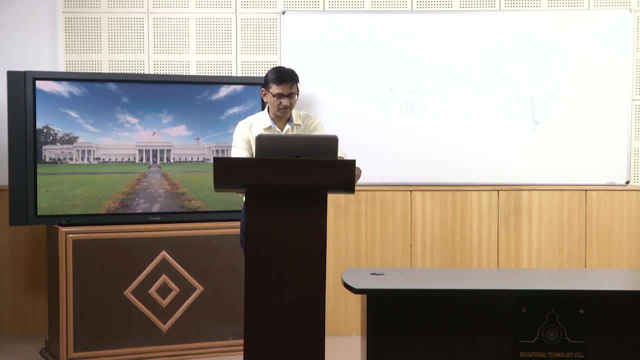 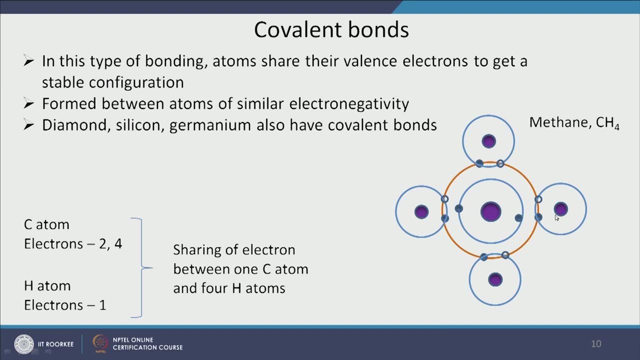 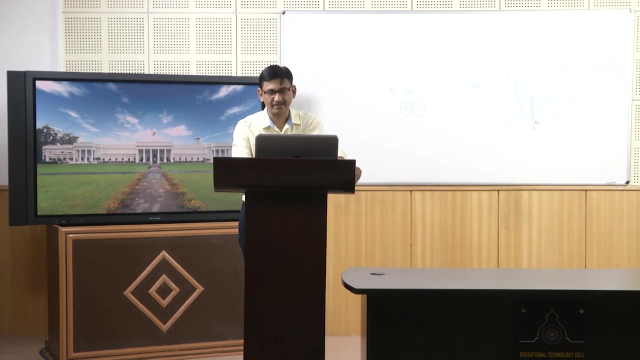 has only one electron, So in one of its shell, the K shell, it needs 2 electron in the K shell. So what it will do, 4 hydrogen atom will combine together, will come together ok, kind of, and they will arrange like this and each hydrogen atom is start sharing an electron with the carbon atom. ok, 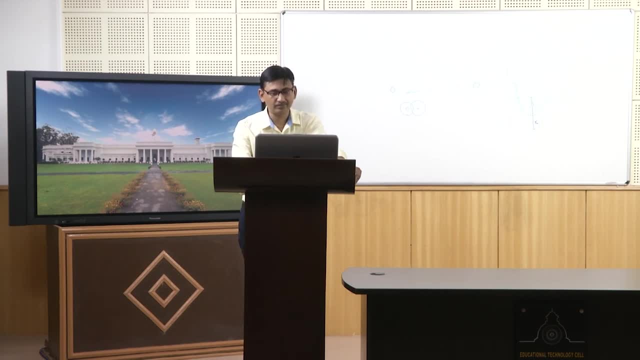 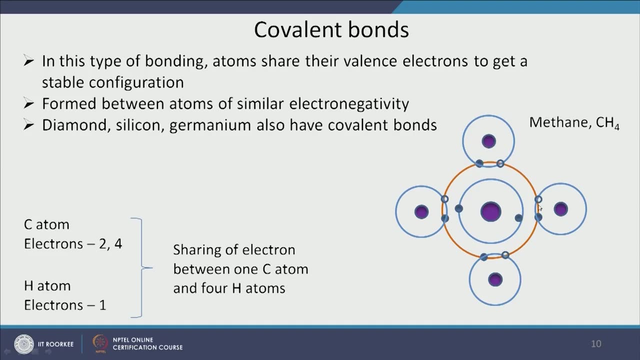 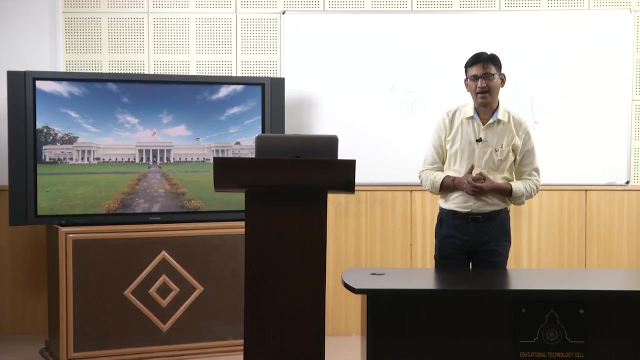 and now hydrogen also has 2 electron- ok. and if you have 4 hydrogen here, the carbon, the L shell of the carbon, also has 8 electrons, ok. So now it is again a very nice situation for both the atoms, ok. So sharing between carbon atom and 4 hydrogen atom will takes. 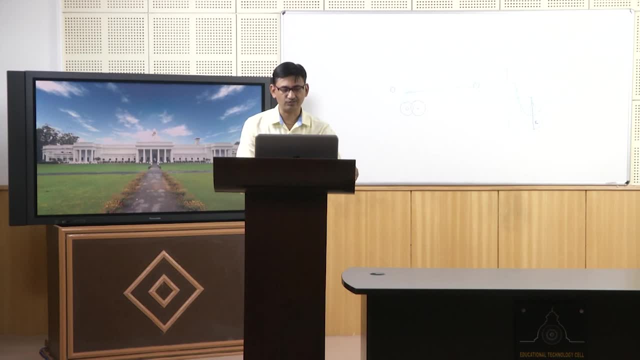 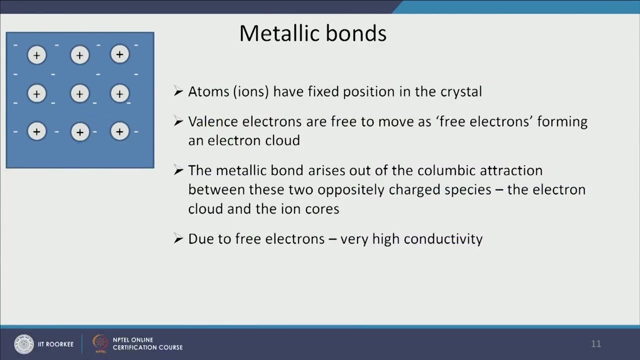 place, and that is what we know as methane, CH4. ok, So this is an example of covalent bond. ok. 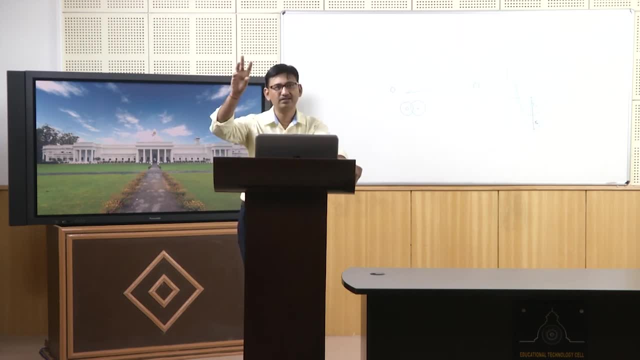 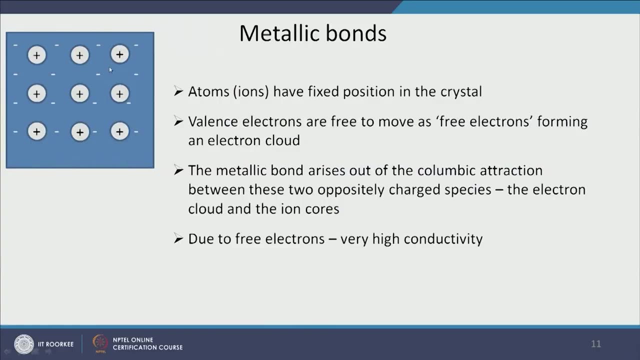 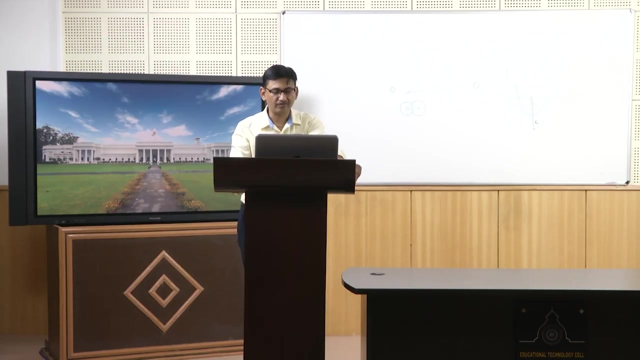 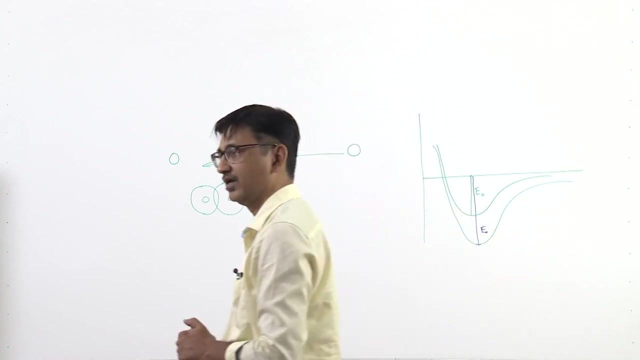 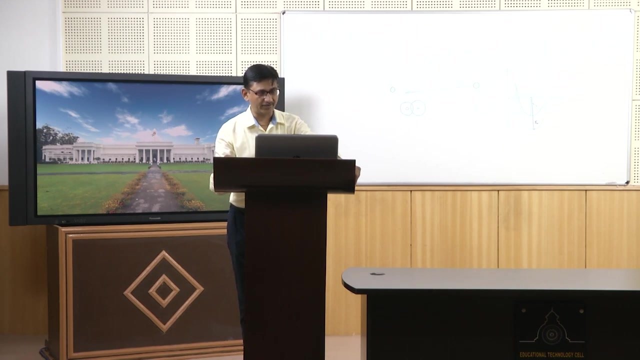 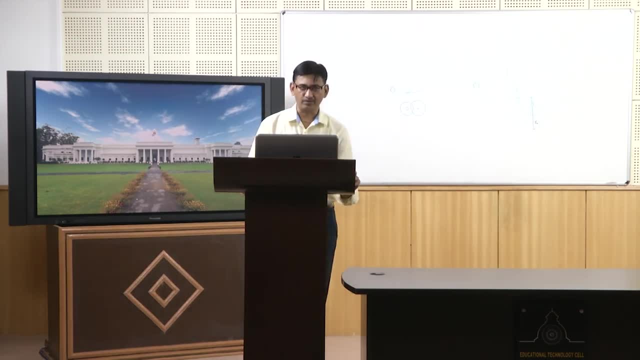 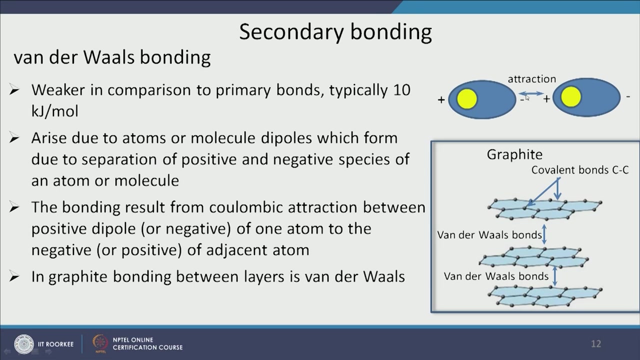 arise due to the formation of a dipole. what happens is that this: there is no symmetric distribution of electron around the nucleus, so because of that it gives you a kind of a charge asymmetry here. so you have a positive charge here, negative charge here. similarly. 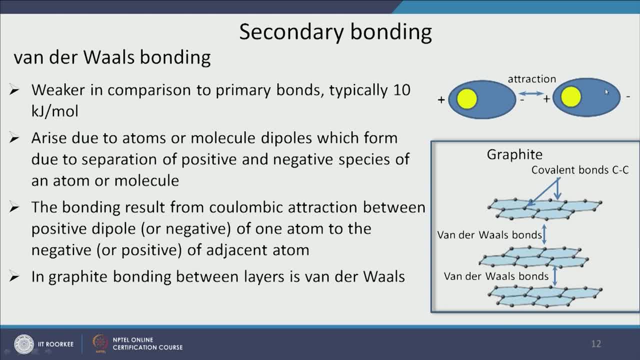 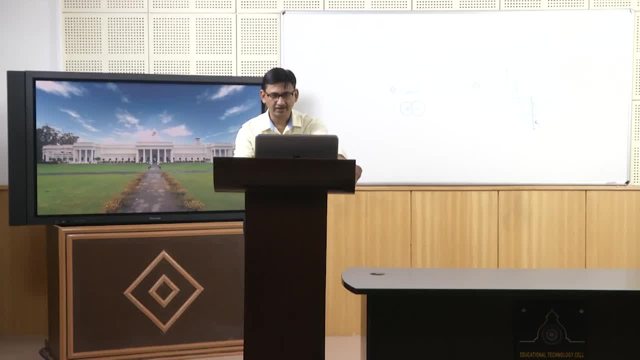 in another atom. also, you will have a positive and negative charged portions in the same atom. So this positive charge and negative charge will interact. again you will have some columbic attraction. attractive forces will be there between these two dipoles and of course this: 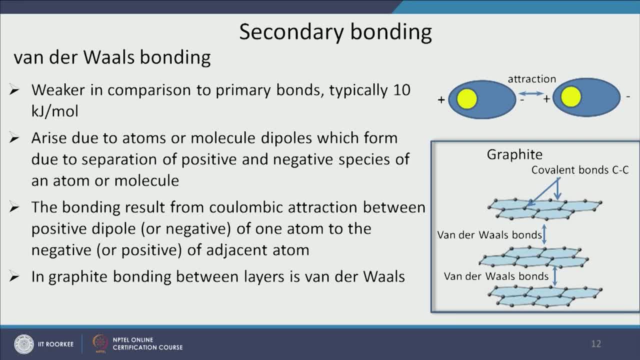 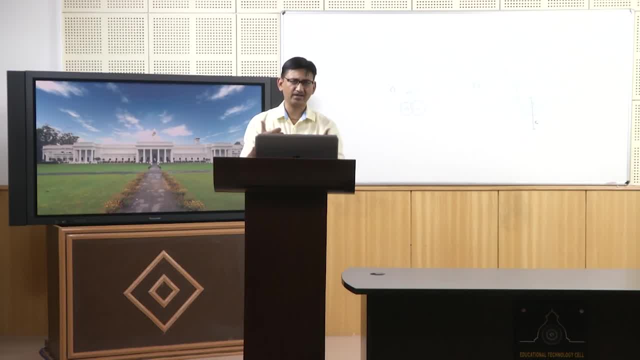 is of not very high. the attraction or the charging is charge on this dipole is not very high, so this bonding is also not very strong. so because of this dipole formation there will be some attraction and they will be. there will be a bond between them, which 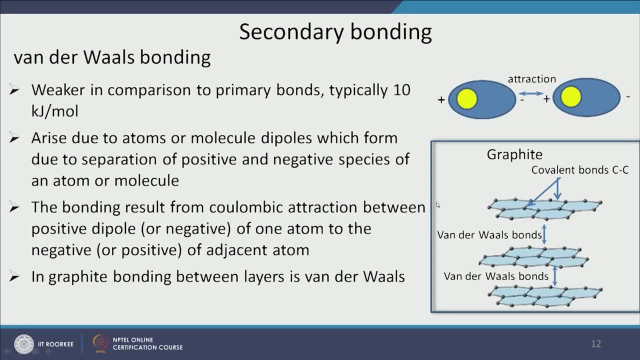 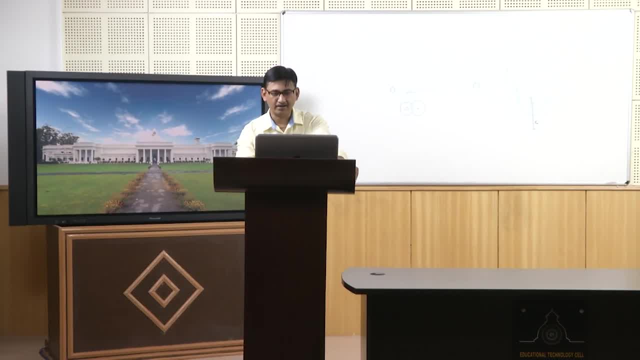 will be called as Van der Waals bonding, In fact in graphite. again I am coming back to the graphite, as we discussed in the first slide also that the graphite has a structure like this: it is in form of layers. so if 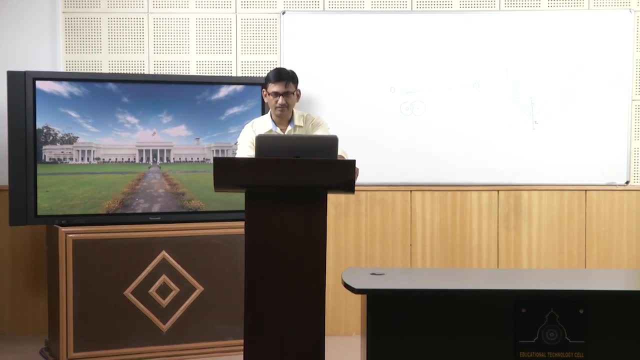 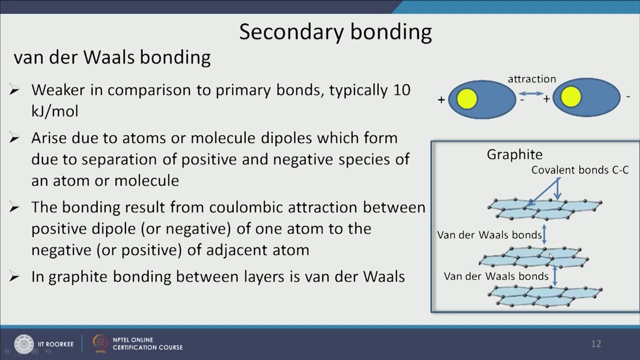 you see, in the layer in plane, the carbon atom have covalent bonds, which is we know are very strong, But between the layers they have Van der Waals bond which again we know are not very strong. So what happens? the covalent bond which is in the plane, those are strong. if so. 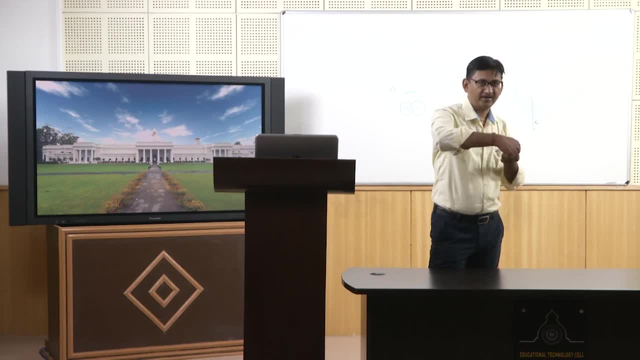 if I deform the graphite in plane, if I do any deformation, you will see that it is. it has very high strength. So if you have one layer over another in graphite, it is very easy because there are Van der Waals bonding only and it is very easy to break them and form new bonds by sliding. 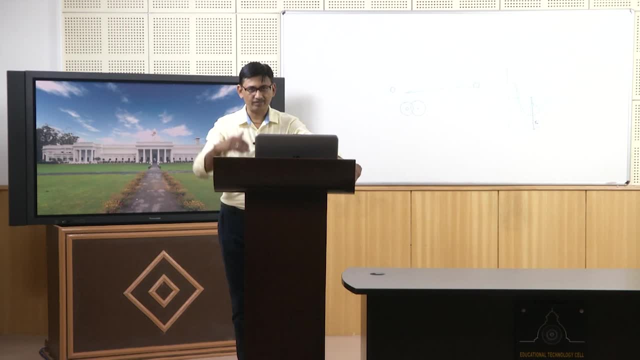 The sliding is very easy in case of graphite because between the layers there is no, there is no primary bond, it is only Van der Waals bond, which are much weaker as compared to the primary bonds. The other type of secondary bond is what we call as hydrogen bonds, and that is what 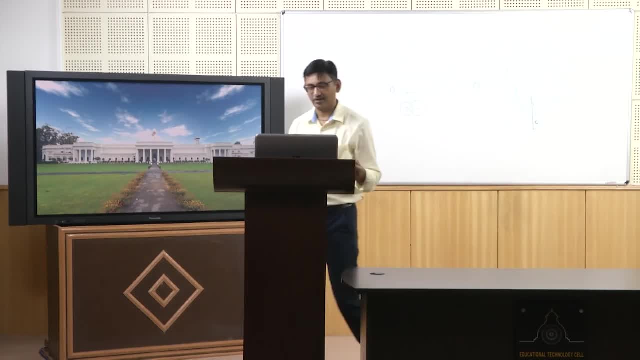 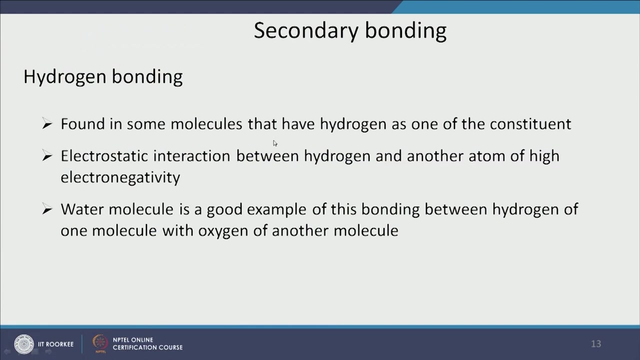 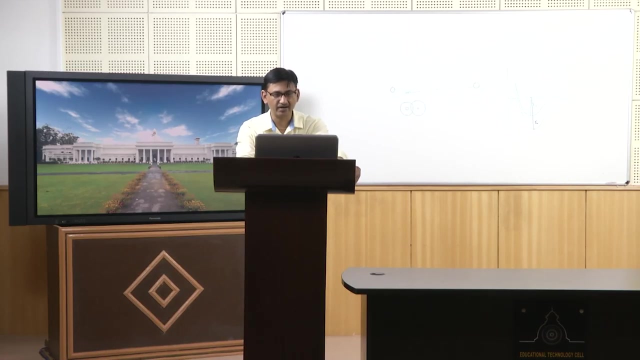 is present in water molecule- water, So water molecule, or H2O, has a hydrogen bonding between the two molecules of H2O. So usually you find this type of bonding in molecules where one of the constituent is hydrogen. The electrostatic interaction between hydrogen and another atom of high electronegativity. 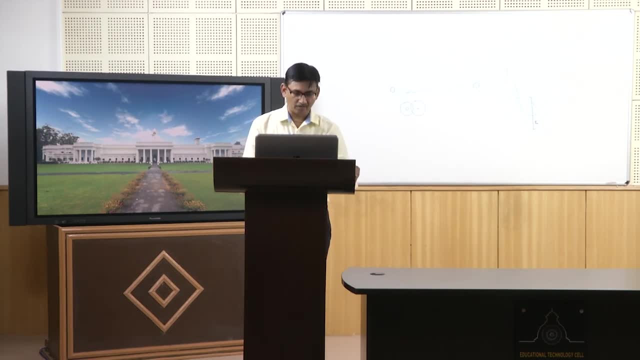 gives this kind of bonding. Water molecule is a good example of this bonding between hydrogen of one molecule with oxygen of another molecule, And that is why it is able to bind together and you can see that water is not easily just separating into molecules. 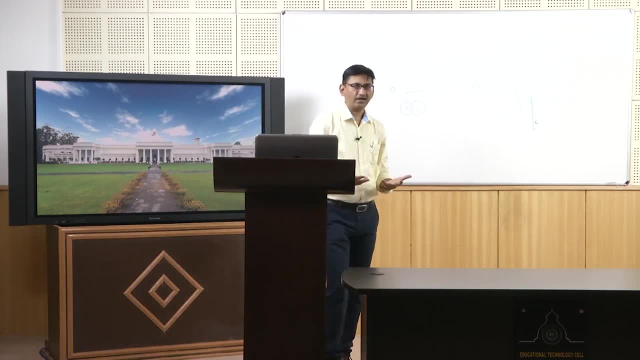 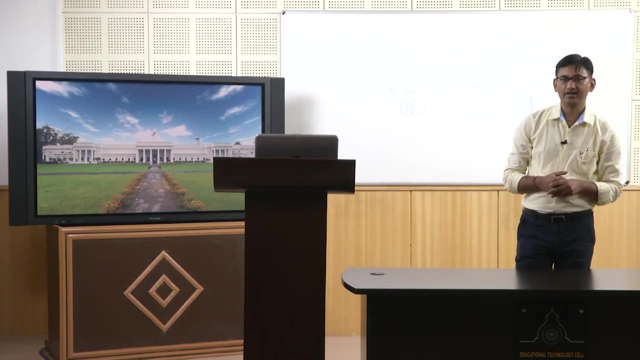 Now, if I want to summarize the all the ideas which we have discussed in this particular lecture, then I can put all this in a nice classification like this, where we have bond type, the strength of these bonds and how these bond affect the properties. So, for example, first we have ionic or covalent bonds. they, these type of bonds, have very high the bond strength is very high. So it is around 450 to 1000 kilo joule per mole and because they have high bond strength they also have high melting point. So you 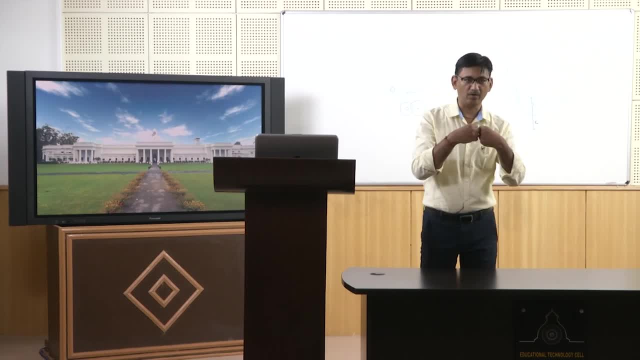 can understand. in solid, the atoms have this kind of bonds. When you want to take it into molten condition or in liquid condition? you want to take it into molten condition or in liquid condition. you want to take it into molten condition or in liquid condition? you? 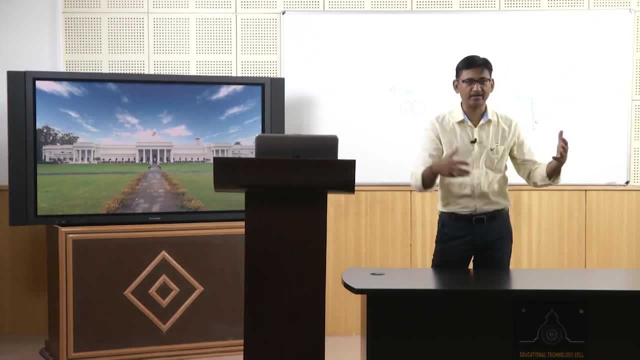 have to break this bond. Then only those atoms in a liquid atoms are can move freely. They do not have any fixed position, whereas in solid they have fixed positions. So for them to move freely in the liquid I need to break this bond. So if the bond strength, is high, it will take more energy to break the bonds. That is why the melting point will be higher. Of course the strength will be higher because you have to first do some kind of stretching. So elastic modulus will be high. the yield strength will be higher because I have to stretch the bonds. So if bond strength is high, the stretching will be difficult. In case of ionic covalent bonds, the atoms are having because of this high bond strength and electrons are shared or interwined with. 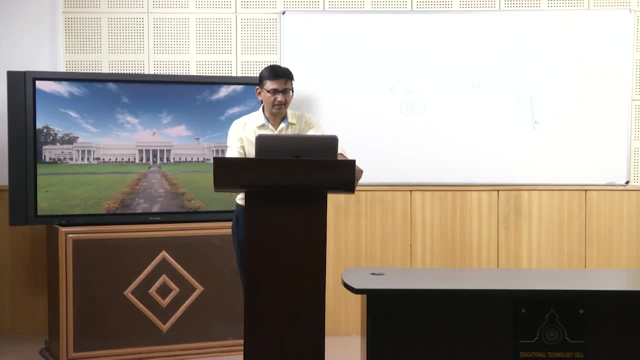 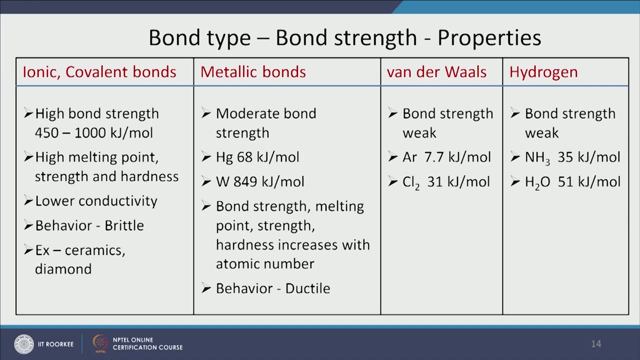 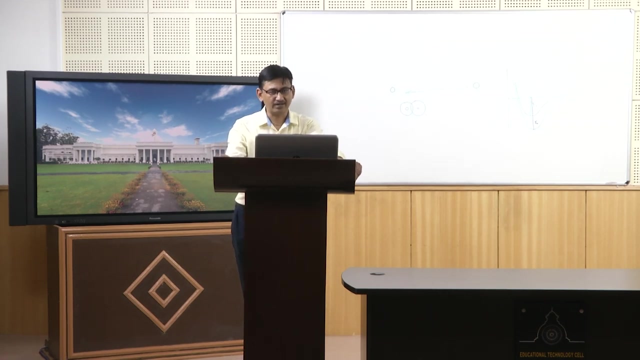 or exchange between the two atoms. it has very low conductivity. electrons are not available for conductivity because it is being shared or exchange between the two atoms. Behaviour is also brittle. right now you may not know this term, but later on, when we will go to mechanical behaviour of materials or the mechanical properties, you will understand. 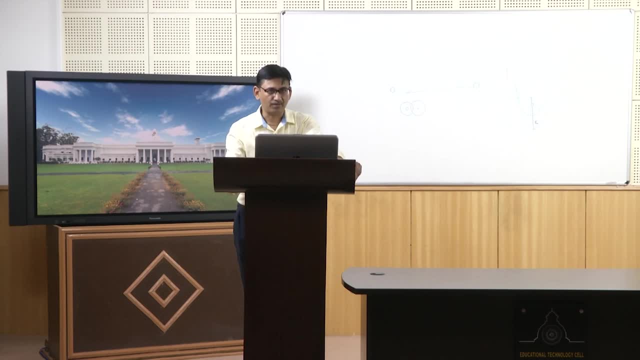 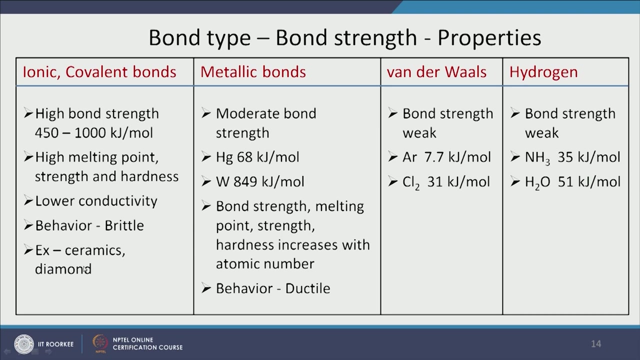 what do we mean by brittle property? but right now you just take it that the behaviour, the mechanical behaviour, or it fails in a brittle manner. for example, this type of bonds you will find in ceramics or diamond. also, diamond has covalent bonds, Metallic bonds. the bond strength is moderate, lower than, of course, ionic and covalent bonds. 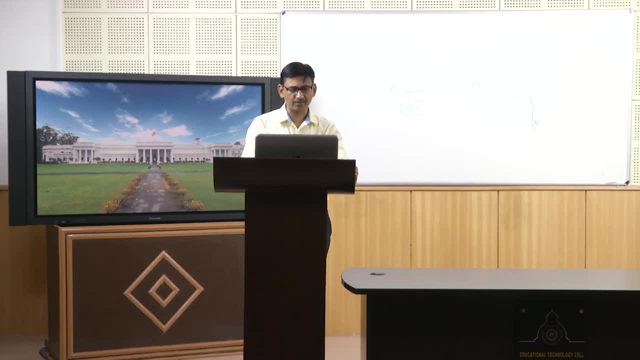 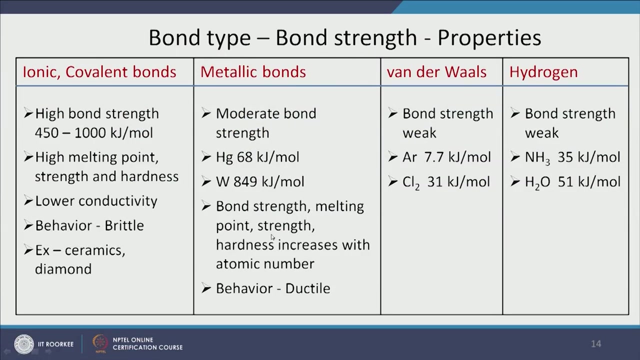 And of course, depending upon the material, you will have different bond strength. for example, tungsten is very high bond strength, very close to what you will find in ionic or covalent bonds. So again, in this case also the bond strength, the melting point, the strength, hardness increases. 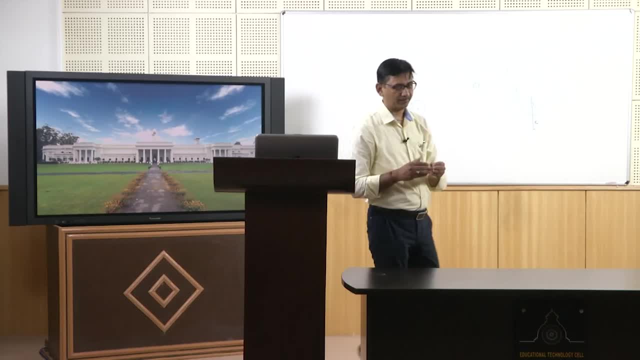 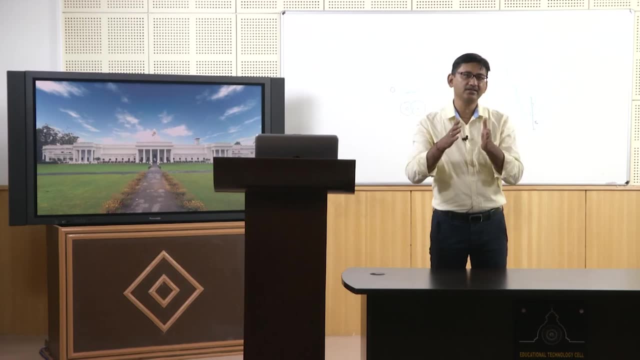 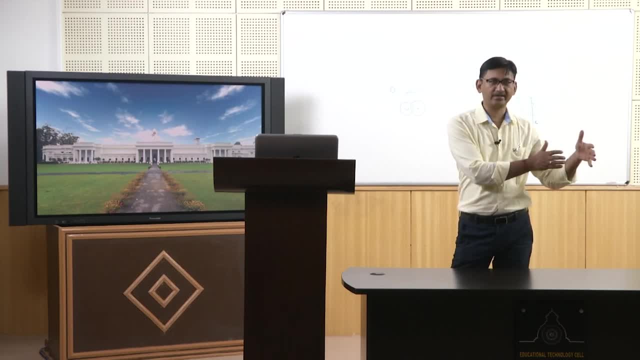 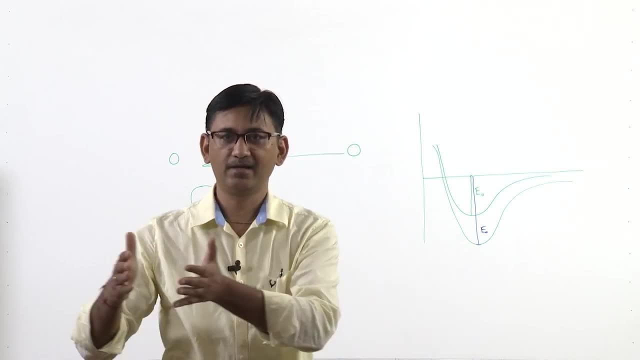 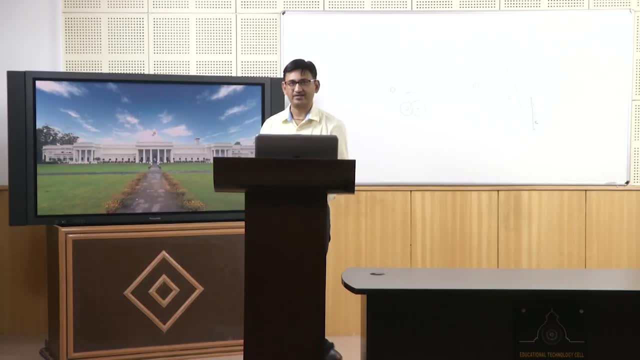 Will Increase, Strength Will Increase And Hardness Will Increase. So It, The Strength, Increases As Function Of this term may be not known to you, but when we will go to mechanical properties, you will.